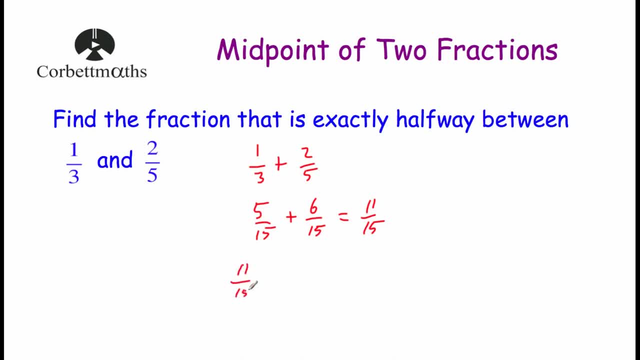 of those fractions. So if we take our eleven fifteenths and we divide it by two, Now remember, two is the same as two over one, So two wholes, that's eleven over fifteen, divided by two over one. And to divide by: 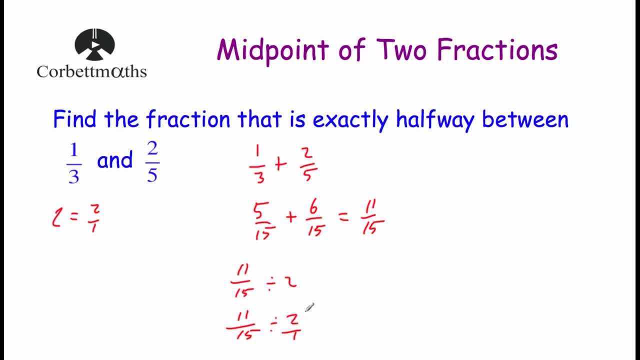 a fraction you can multiply by the reciprocal. So the reciprocal is what we find when we flip over the fraction. So that's going to be eleven over fifteen multiplied by one over two. Eleven times one is equal to eleven, and fifteen times two is equal to thirty. 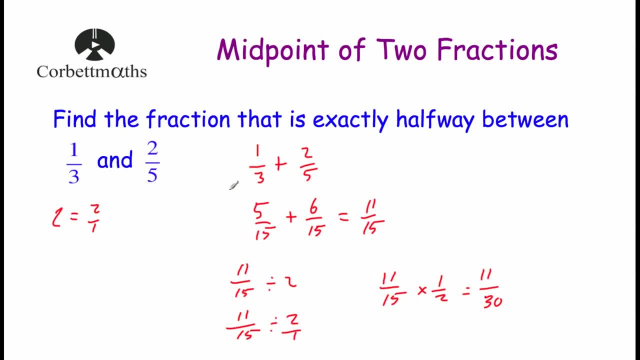 So the fraction that is exactly halfway between one third and two fifths would be eleven, thirtieths, and that's it. Okay, let's have a look at another question. So our next question says: find the fraction that is exactly halfway between one half and. 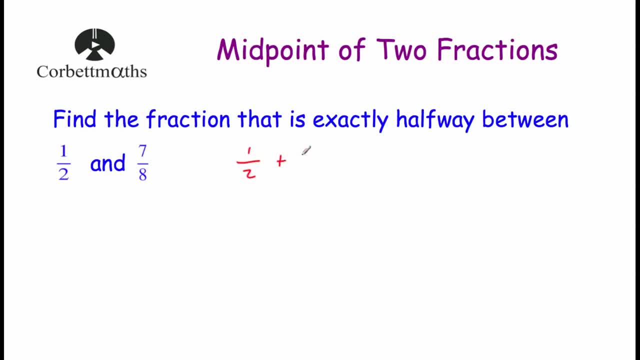 seven eighths. So again we're going to add the two fractions together, the one half and the seven eighths. So our denominators are two and eight. So the lowest common multiple of two and eight is eight. so let's have eight on the denominators. Seven eighths will just be seven eighths. 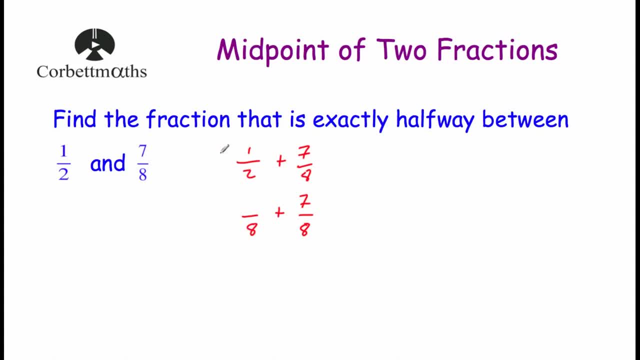 To get from two to eight, we multiply by four. so we multiply the numerator by four. So one half is four eighths. Now, adding those two together, the four eighths and the seven eighths will be four plus seven is eleven. 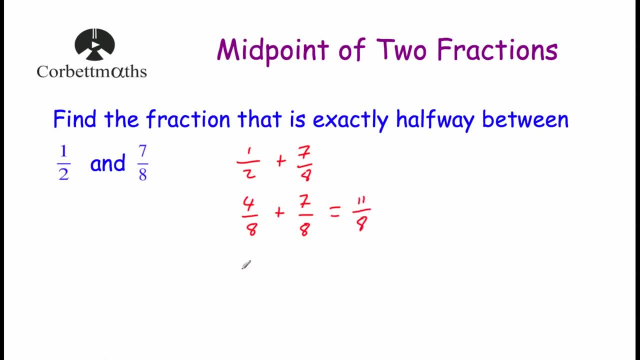 Now we need to divide this by two, so it's going to be eleven over eight divided by two over one, and that would be the same as eleven over eight multiplied by one half, and then that would give us: eleven times one is equal to eleven, and eight times two is equal to. 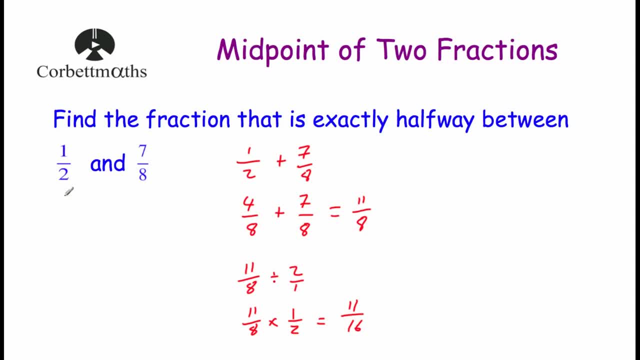 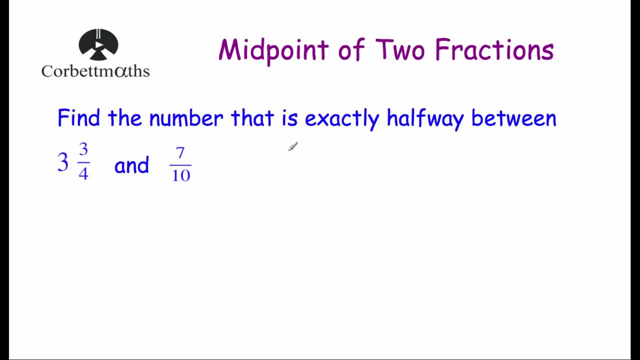 sixteen. So the fraction that is exactly halfway between a half and seven eighths would be eleven sixteenths, Right? so let's have a look at our last example. So our last question says: find the number that is exactly halfway between three and. 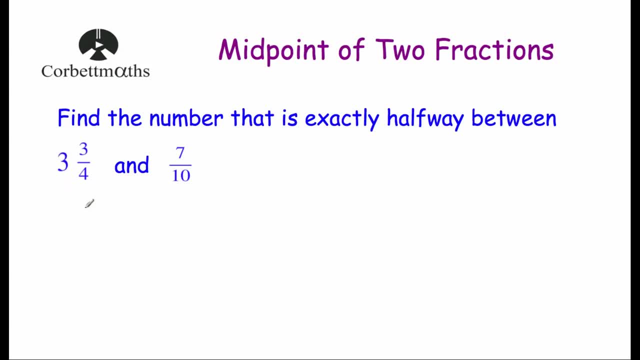 three quarters and seven tenths. So you might notice that three and three quarters is a mixed number. so let's change that into a top heavy fraction. So three times four is twelve plus three is fifteen, so that would be fifteen quarters. 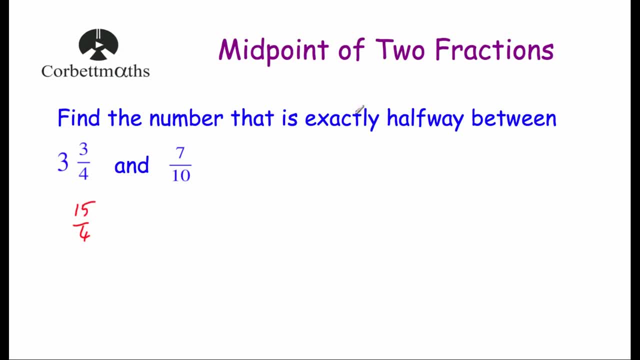 So three and three quarters is the same as fifteen quarters, And we want to find the number that is exactly halfway between fifteen quarters and seven tenths. So we'll add these two together, so fifteen quarters plus seven tenths. So we want to find the common denominator of four and ten. well, I think twenty would be a good number.